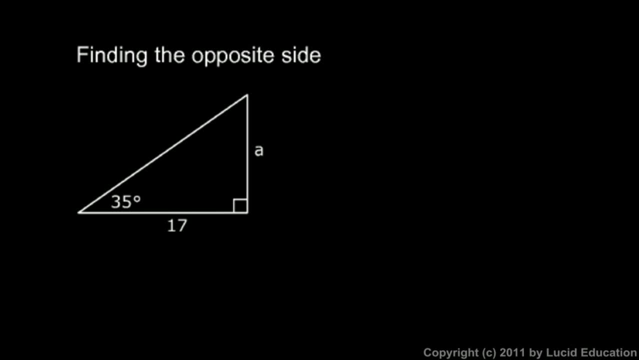 and this side over here that is opposite. the 35 degree angle is unknown, So we've just named it with a variable, a in this case, and we know the adjacent side that's given is 17.. So we know this. we know that the tangent of any angle is the length of the opposite side divided by the length. 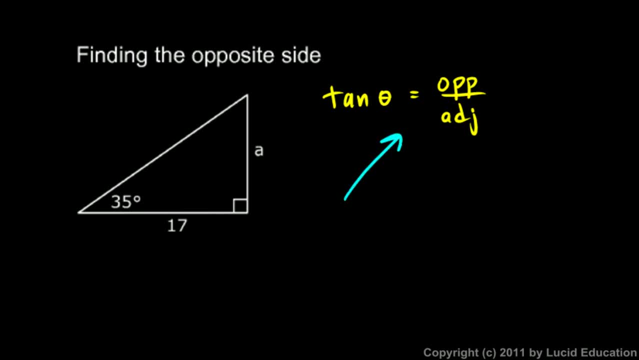 of the adjacent side. What you want to do is just take that concept and apply it in this situation. So the tangent of an angle is the opposite over the adjacent. That means the tangent of this angle has to be this length over that. I'll say that again. That is the mental step of setting up the 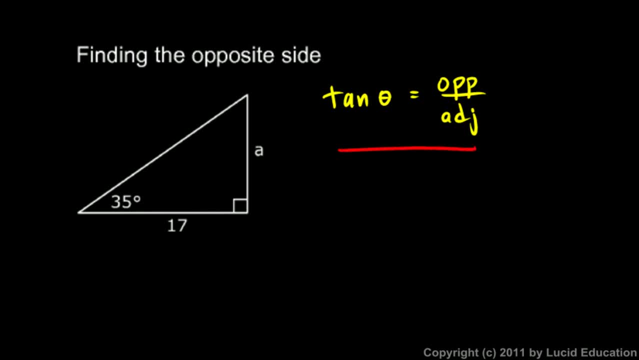 problem, and that is most of the battle here. We know that the tangent function or the tangent of an angle is always the length of the opposite side over the adjacent side. So right here, the tangent of this angle has to be this length: the opposite over the adjacent. So let's write that: 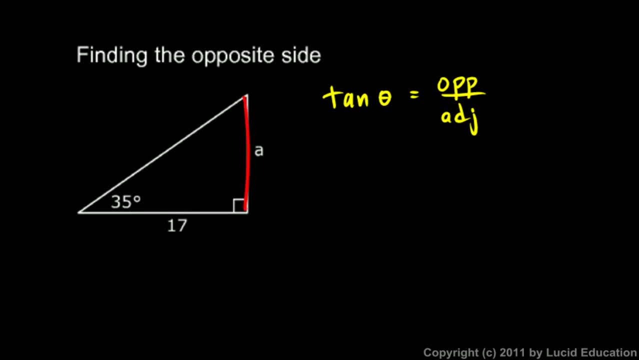 mathematically, I'm going to write, the tangent of this is equal to this over that. So in this particular case, that means this: The tangent of 35 degrees is equal to a over 17, and we can solve this for a. You should be able to do this mentally without writing it, but I'm going to write it. We. 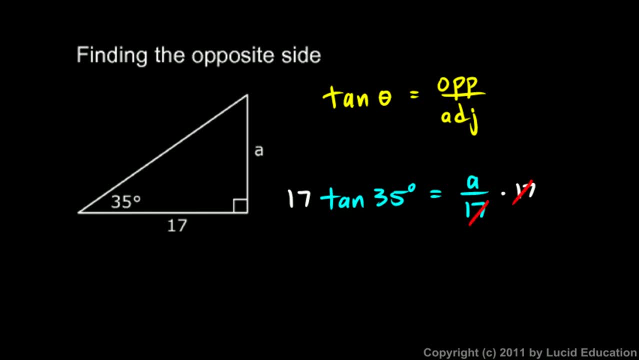 multiply both sides by 17 and the 17s cancel, and we're left with with a is equal to this. So I'll write: a is equal to 17 times the tangent of 35 degrees, and again you should be able to go from here to here mentally. So a is 17 times the tangent of 35 degrees. This you can do. on. 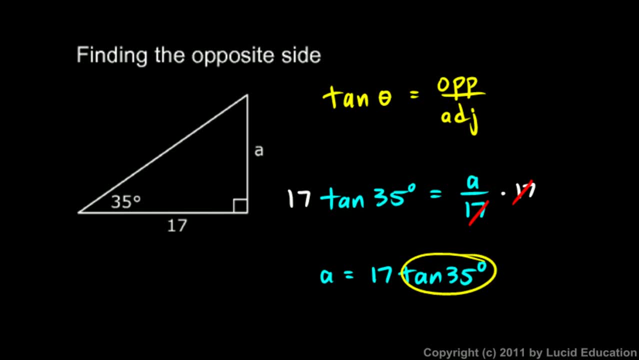 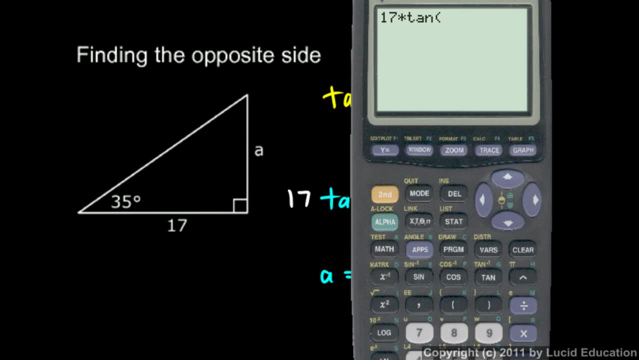 the calculator, because the calculator can give you a value for the tangent of 35 degrees. So we pull up the calculator and we say 17 times the tangent of 35, and this will be the answer, 11.9, and you have more decimal places there, but we'll round it to. 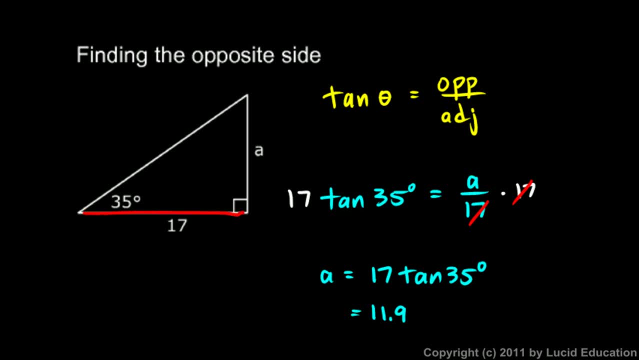 11.9.. So that's the answer. If this length is 17 and it's a right triangle and that angle is 35, then this side has to be 11.9.. Now here's a similar example, but this time we will.